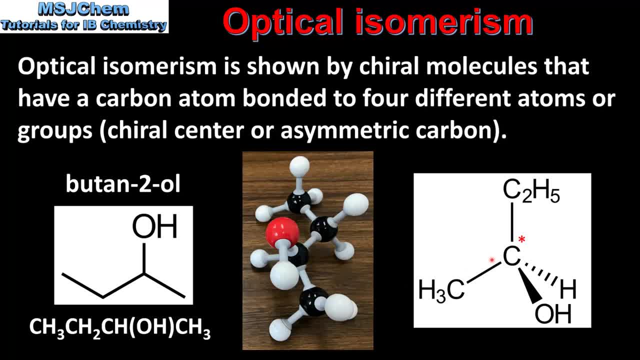 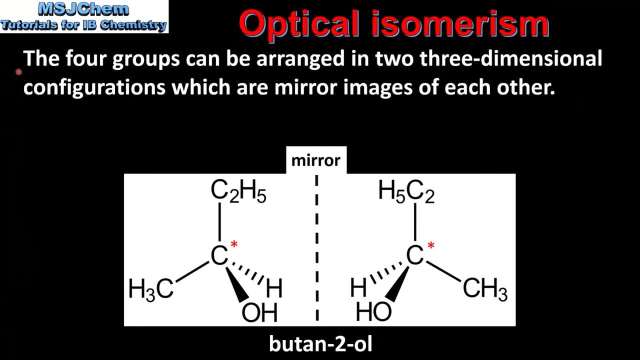 On the right we have the stereochemical formula of butan-2-ol. The asymmetric carbon is marked with a red asterisk. The four groups around the chiral center can be arranged in two three dimensional configurations which are mirror images of each other. The two mirror images are non. 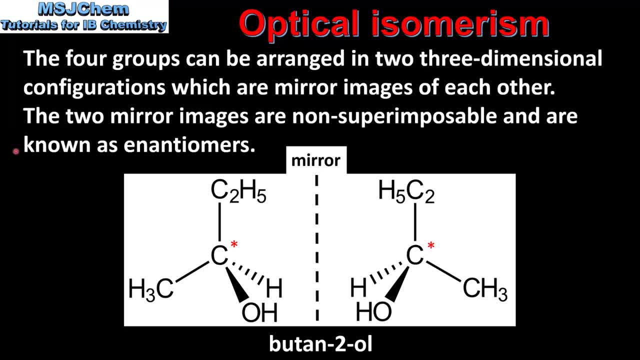 superimposable and are known as enantiomers. So here we can see the two enantiomers of butan-2-ol. As you can see, the enantiomers are non superimposable and are known as enantiomers. 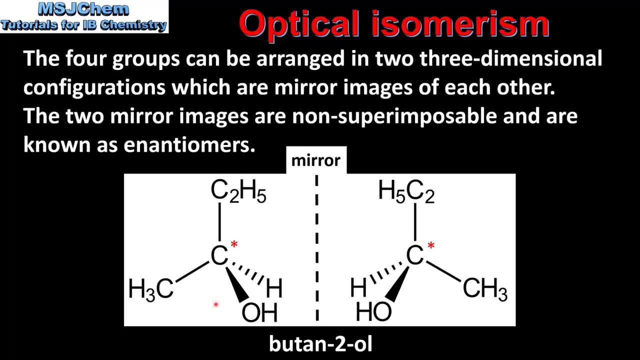 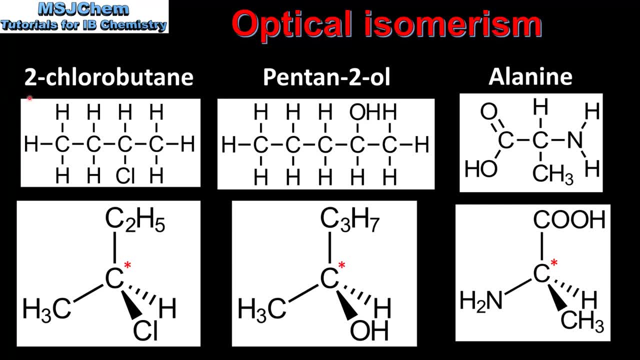 So here we can see the two enantiomers of butan-2-ol. As you can see, they are mirror images of each other and non superimposable. Next we look at some more examples of chiral molecules. From left to right we have 2-chlorobutane, pentan-2-ol and the amino acid alanine. 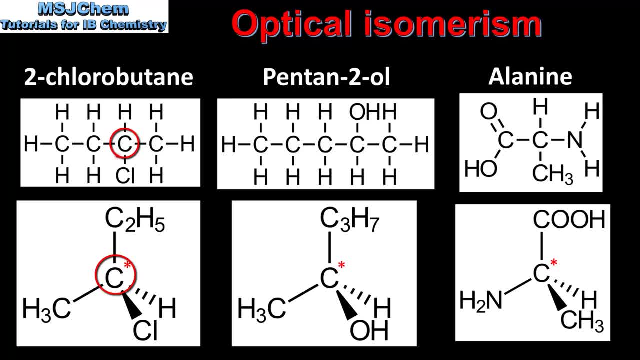 If we start with 2-chlorobutane, we can see that this carbon atom is bonded to four different atoms or groups. Therefore, it is an asymmetric carbon. In pentan-2-ol, we can see that this carbon atom is also bonded to four different atoms or groups, And in alanine, this carbon atom is also. 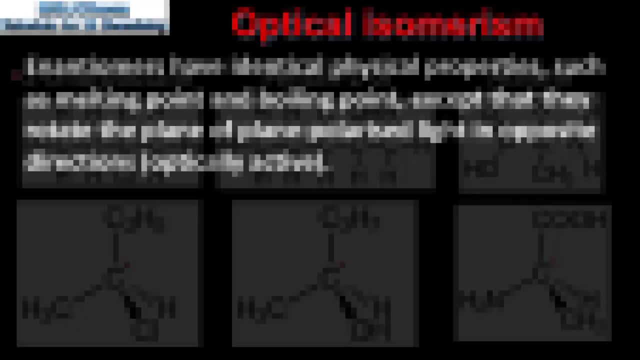 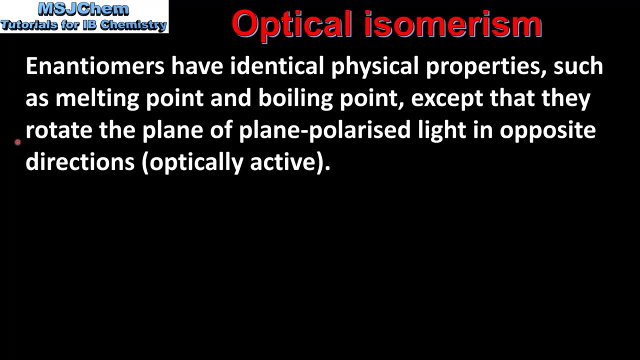 bonded to four different atoms or groups. Enantiomers have identical physical properties, such as melting point and boiling point, except that they rotate the plane of plane polarized light in opposite directions, which means they are optically active. This property is used to distinguish between the two enantiomers of a chiral molecule.